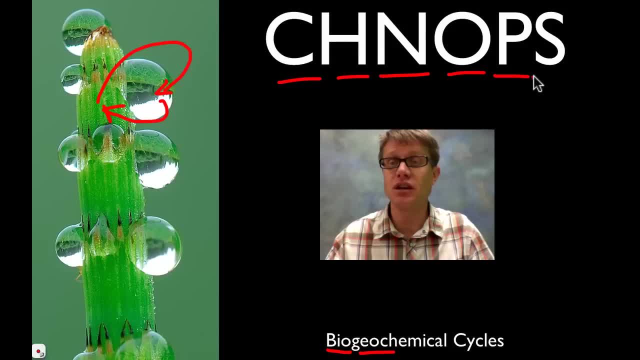 back again, And so up here I've written this, which is just a mnemonic device to remember the atoms that life needs to survive. schnapps, And it's carbon, hydrogen, nitrogen oxygen, phosphorus and sulfur. And so before we actually talk about cycling, let's talk about why we 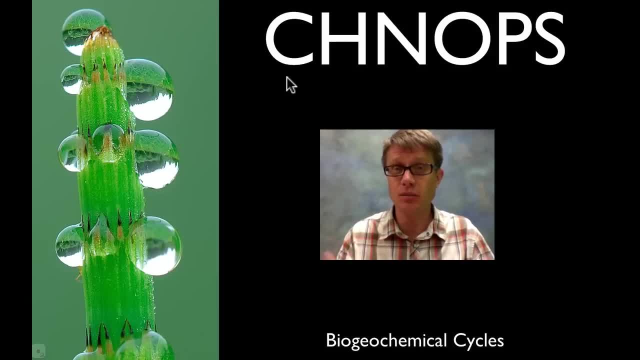 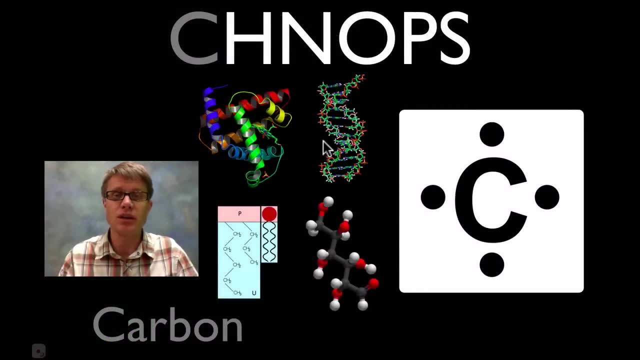 actually need these atoms And we're going to start with carbon And try to be ahead of me. In other words, before I flip the slide, you should be planning ahead. Why do we need carbon? Why do we need hydrogen? So let's go to carbon. So why do we need carbon? Well, 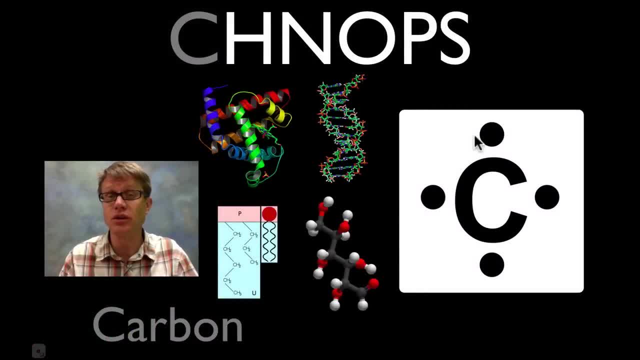 carbon, remember, has four valence electrons, So it's really good at bonding And so it's good at making complex organic materials And so, basically, if you're thinking of a protein or lipids, or carbohydrates, or nucleic acids like DNA, all of these things are built out of carbon, And that's because carbon is. 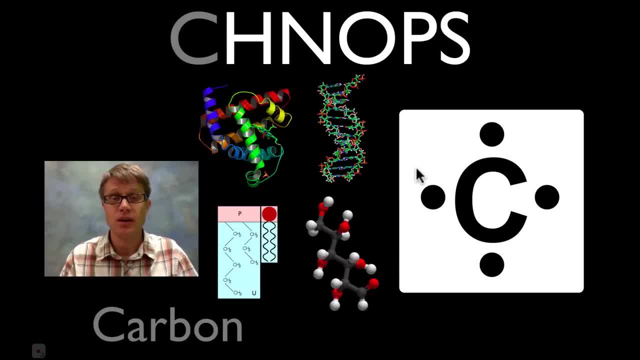 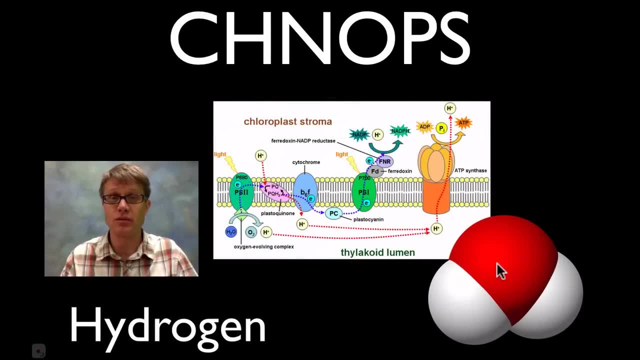 incredibly good at building upon itself. If we go to the next one, why is hydrogen important? Hydrogen is important because it makes up water, And water in general is important just because of its solubility And it can provide a medium where life can exist, But it also 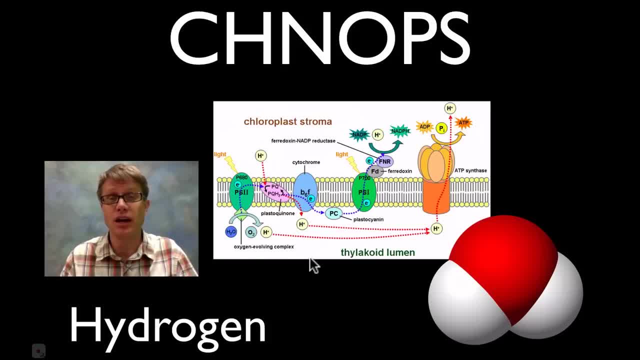 can provide energy. Look here: This is the light dependent reaction in photosynthesis, And you can see these protons, as they flow through ATP synthase, are actually making energy in the form of ATP, And so hydrogen is important, just through water, but also energy transfer. So be thinking ahead. Why do we? 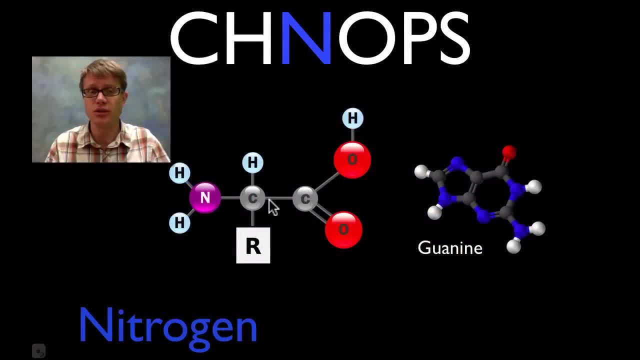 need nitrogen. Well, nitrogen we need for a couple of reasons. This right here is an amino acid And remember, DNA contains the blueprint to make life, But it's the proteins that actually make us the way we are. So, it's the proteins that actually make us the way we are, And 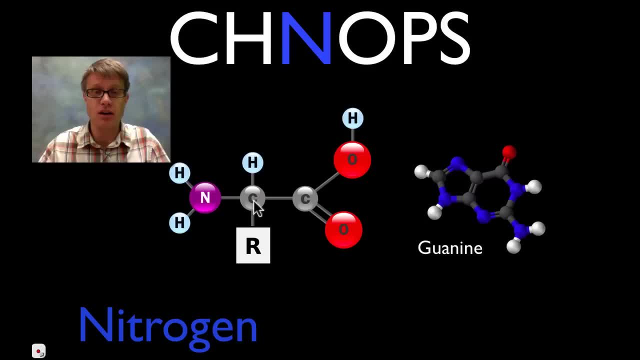 this right. here is an amino acid. All amino acids are going to have a carbon in the middle and a hydrogen attached to that. They're then going to have an amino group on one side and a carboxyl on the other side, And then an R group. That's going to be the difference. 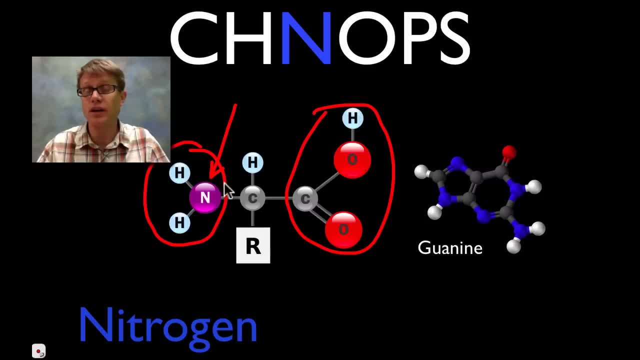 in every amino acid. But this nitrogen right here is required to make amino acids or to build proteins, And so we need that nitrogen to survive. This over here is guanine. Where's guanine found? Well, when you're talking about DNA, what's in the middle? in other words, 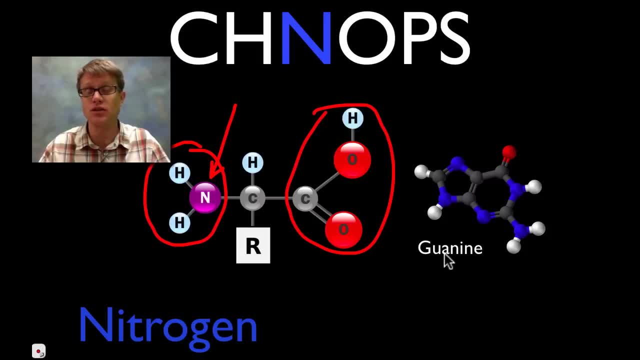 what stores the information are the nitrogenous bases, And the nitrogenous bases are the nitrogenous bases And the nitrogenous bases are the nitrogenous bases And the nitrogenous bases are the nitrogenous bases. Guanine is just one, But we also have cytosine, thymine and adenine, And so guanine. 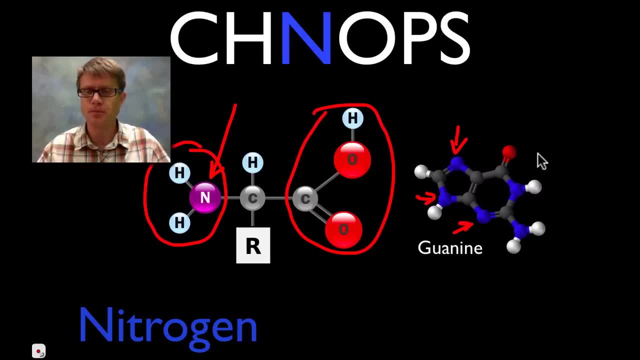 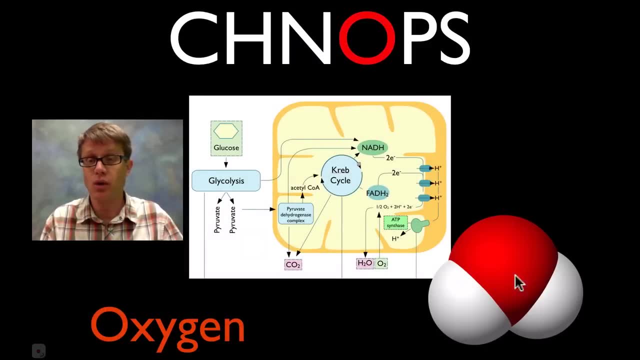 if you look here, has a whole bunch of nitrogen in it, And that nitrogen we have to get from our atmosphere just to make the genetic material. Let's go to the next one: Oxygen. Why do we need oxygen? Well, water, of course we need oxygen for, But I also included cellular respiration. 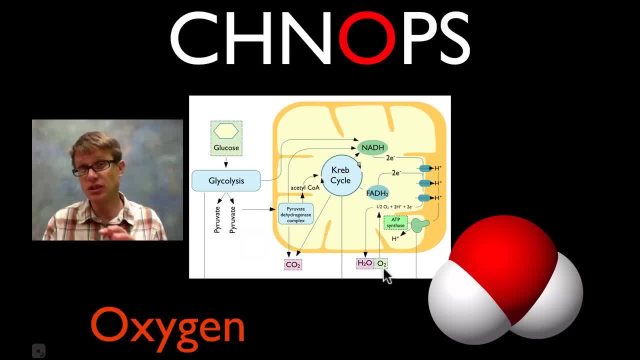 here, Because way at the end of cellular respiration, oxygen is receiving those electrons, And so we can get a huge amount of energy as those electrons fall to oxygen. Likewise, when we pull them away in photosynthesis, we can store a lot of energy If we go to the. 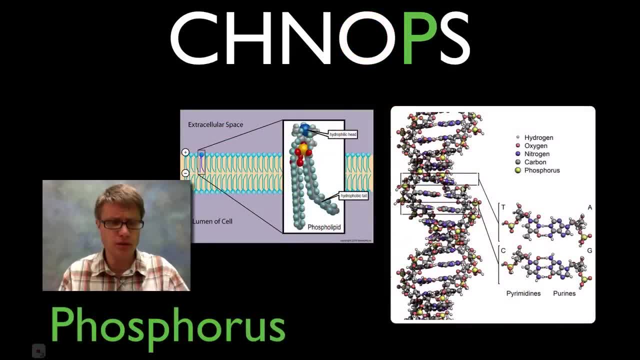 next one: phosphorus. Why do we need phosphorus? Well, we need phosphorus for a few reasons. Number one: this would be a phospholipid That makes up our lipid bilayers And it's going to have a phosphate in its head. If we look on the DNA right here, on the DNA, we're 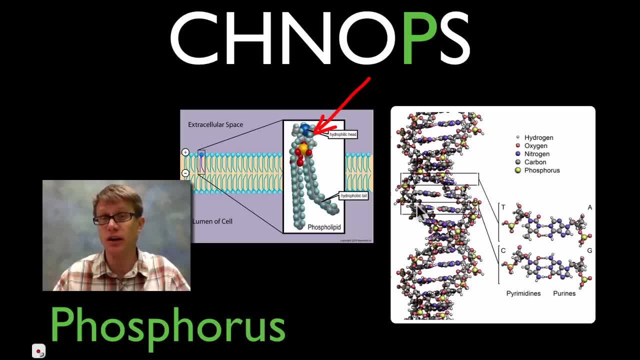 going to have, remember, sugar, phosphate, sugar, phosphate, sugar, phosphate, backbone, And so phosphorus is important in making our nuclear material, And the one thing that I should have included on here is 18.. And remember, ATP is adenosine triphosphate, And as we attach that last phosphate on, we're 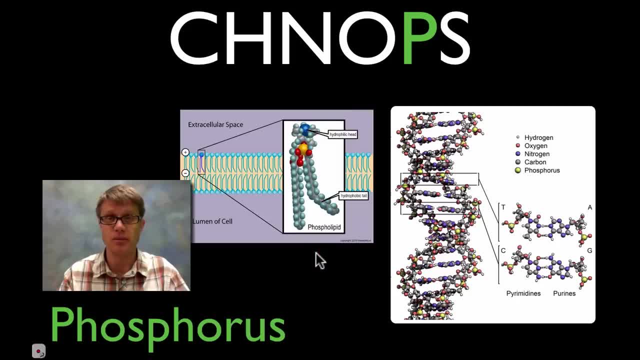 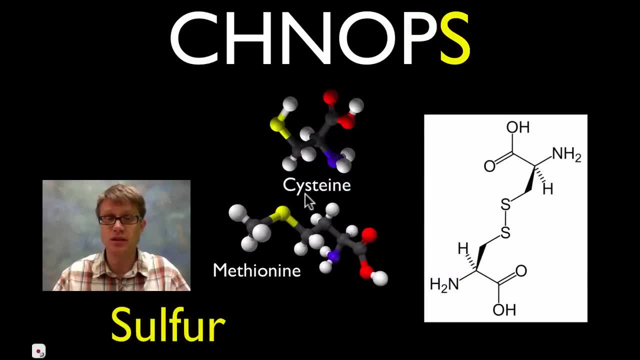 storing energy. Likewise, we can release energy as we let it go. One of the hardest ones here is sulfur. Why do we need sulfur? Well, if you look right here, I've got two amino acids. This is cysteine and methionine. So we just learned what an amino acid is. Again, it's. 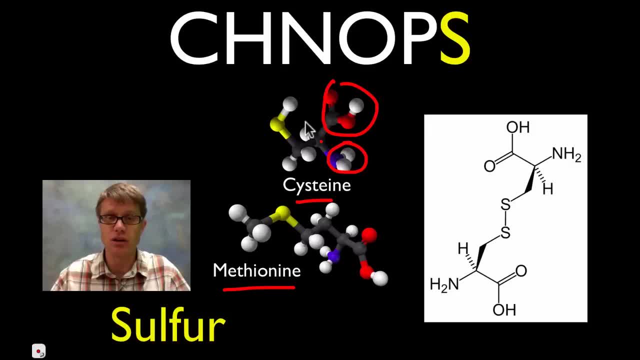 going to have its carboxyl group. here It's going to have its amino group, its carbon and its hydrogen. But you can see, in both of these amino acids we're going to have sulfur. And why is sulfur important? Well, remember, proteins make us the way we are. 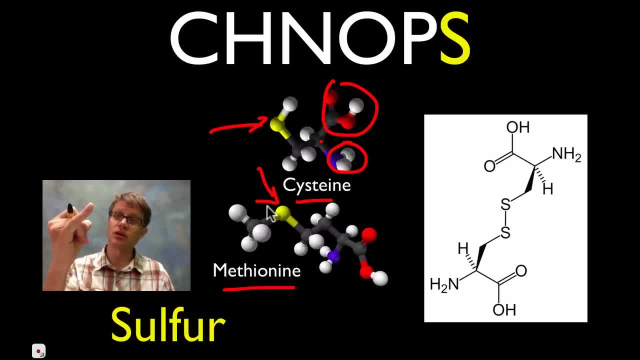 And they have this complex three dimensional shape And basically, if you have a sulfur and a sulfur in two R groups, they'll be held together with a bond And this is called a disulfide bridge or a disulfide bond. And so sulfur is important because it gives us 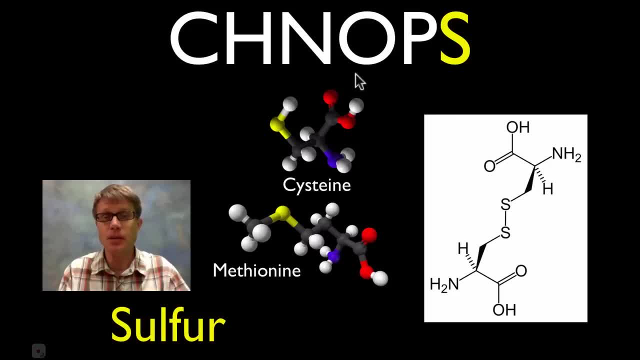 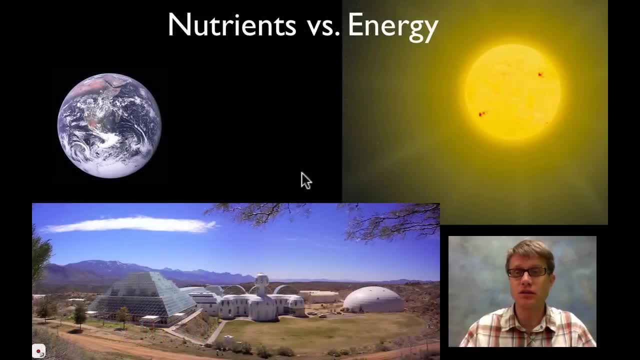 structure to those big proteins, And so schnapps is a good way to remember all the things that we need. And again, we need them for various reasons, And so we have to get them from our environment. Let's talk about energy. How does energy get from the sun to the earth? It just travels. 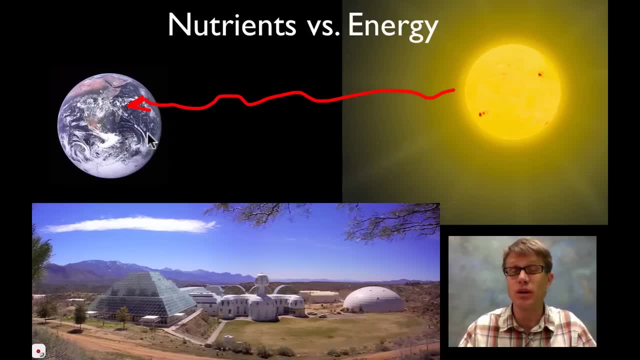 as light. Once it gets to the earth, it's eventually used, But it also eventually ends up being given off as something called heat, And so the way that energy gets to our planet is one direction. It's going to move in one direction Then it eventually ends up as heat, But the 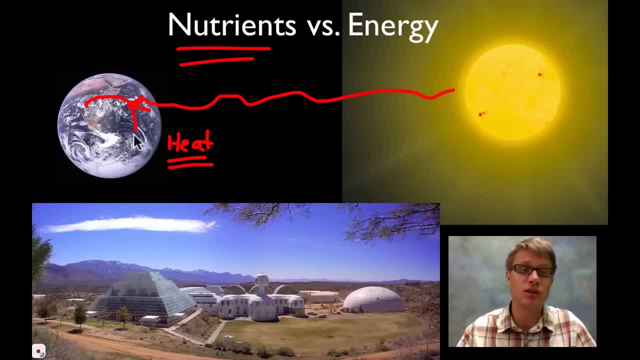 nutrients on our planet are different. The nutrients on our planet are going to be recycled. In other words, the amount of water that we have on our planet is static. The amount of carbon that we have is static, And it has to be recycled over and over again, And that's. 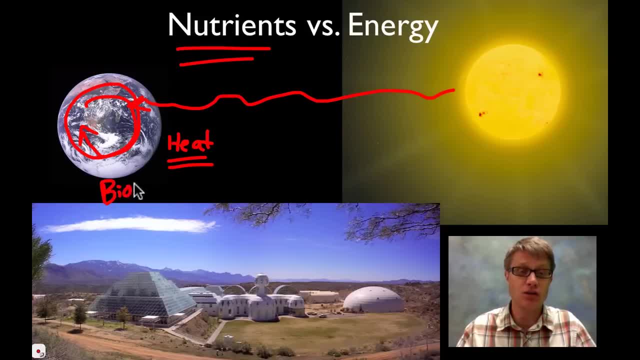 going to be recycled over and, over and over again on biosphere, which is the earth, And they tried to do this in the Arizona desert where they built this, which is biosphere 2. They tried to keep all the nutrients inside this biosphere that they needed to survive. 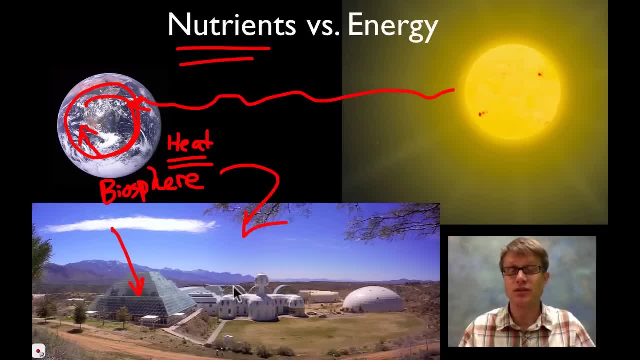 They let light in, but they tried to recycle the nutrients. It worked okay. They didn't really get a good balance, and so they had to open it up occasionally, And so there are cycles by which we can return that from life to non-life and then back again Remember. 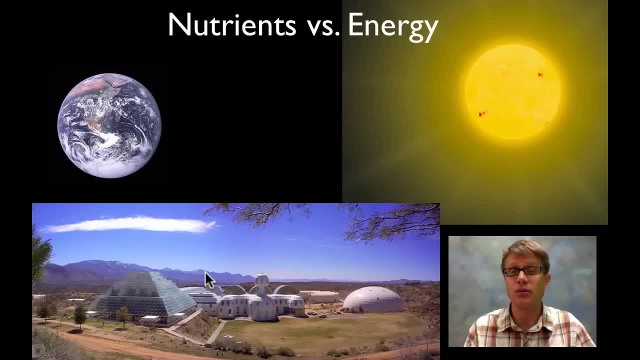 what we're talking about is biogeochemical cycling. How do we go from living to nonliving, And so on the next four slides. what I want you to think about is, with each of these cycles from the water to the carbon, to the nitrogen, to the phosphorus, where is most of that nutrient? 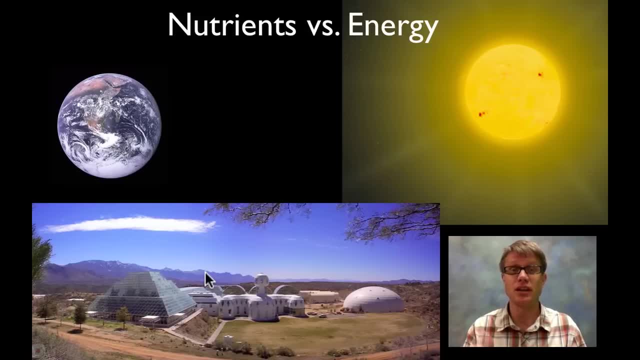 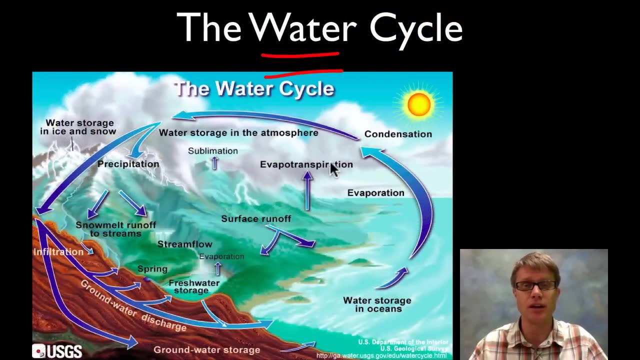 stored? How does it get into plants, And then how does it get into animals, And then how does it get back again? So let's start one with one that we all know, So the water cycle. So where is most of the water stored on our planet? It's going to be stored in the ocean. 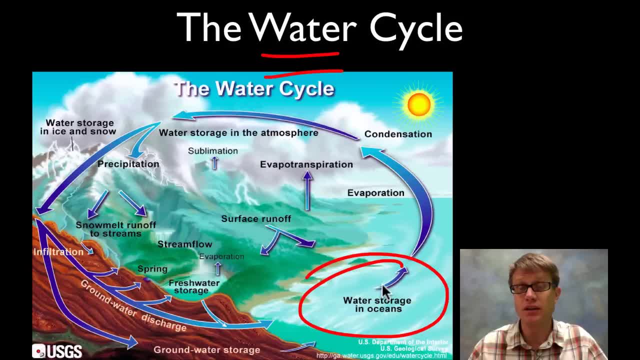 And so that's going to be the reservoir, That's going to be where most of the water is. How does it get into plants? Let's start there. Well, there's evaporation, condensation, precipitation, But eventually we have to get it into the plants And it's going to move. 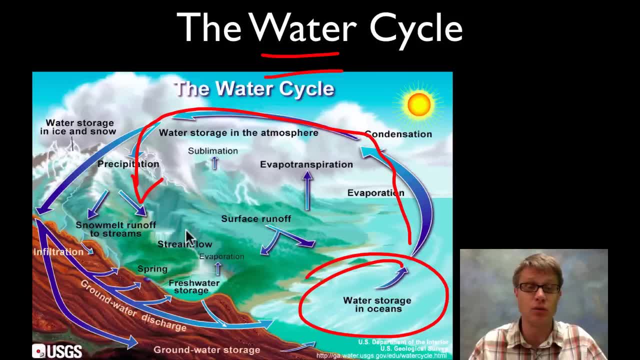 into the plants through their roots. They're going to absorb that water. It's going to move up through the xylem, So that's how it gets into plants. How does it get into animals? Well, we get water in us by drinking it Or eating plants that contain water. How do we? 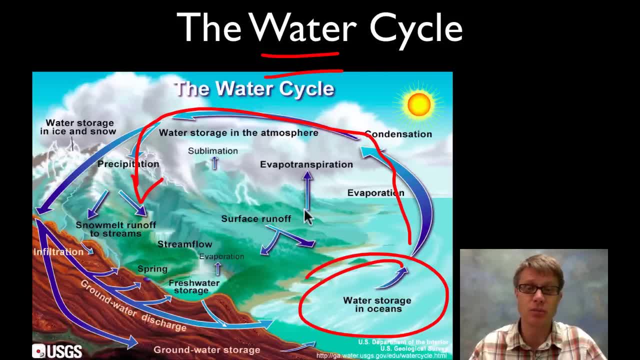 lose it. In other words, how does it go back to the reservoir again? Well, if you look at it's plants, we're going to transpire. They're going to lose that water through their leaves And in us, just sweat or urination. we're going to lose that water back to the environment. 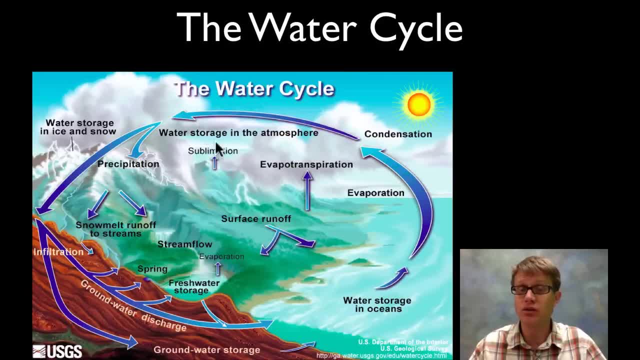 so it can be recycled again. And so the water in a water bottle used to be water in an ocean, It used to be water in a plant, It used to be water in a swamp. It's just recycled over, and, over, and over again. So that's the water cycle. Let's go to the next one, That's the. 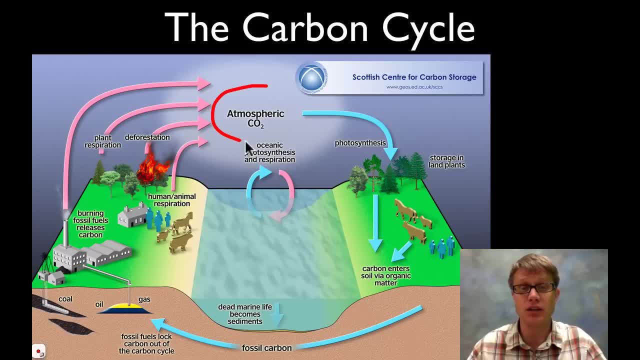 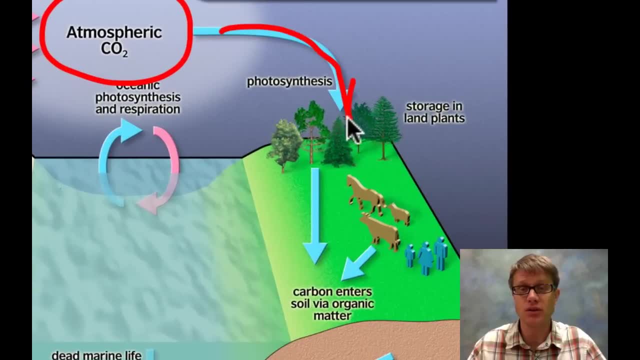 carbon cycle. Where is most of the carbon stored on our planet? It's actually stored in the atmosphere. So how do we get that water back into the environment? Well, we're going to have to get that into plants. We get that into plants through photosynthesis. Again, they're going. 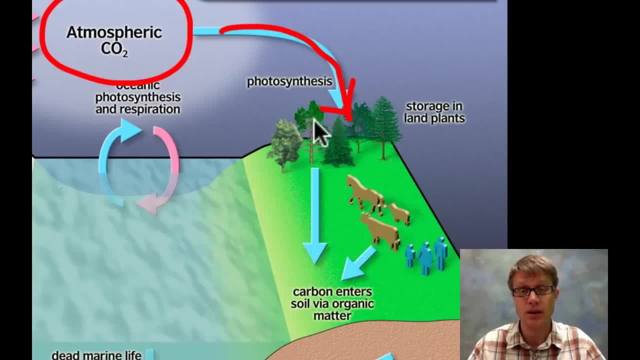 to absorb carbon through their stomata and make sugar out of it. Okay, So how do we get it back to the environment? Well, how do we get carbon? We're going to eat plants, Or we're going to eat things that eat plants, And so that's how we get carbon inside us. 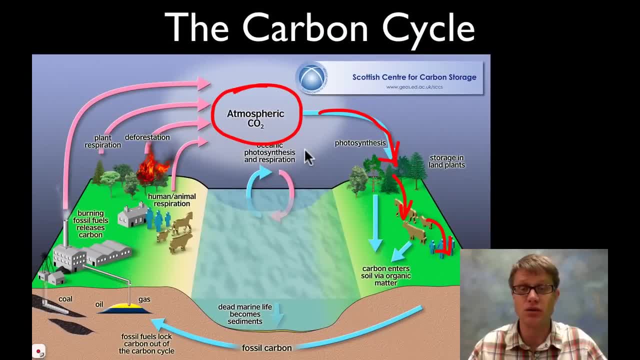 But how do we then return it back into the atmosphere? We're going to do that through respiration, And so as we respire, we're going to return that. As plants respire, remember they're doing respiration as well. That returns it. Now, one thing that we're changing: the 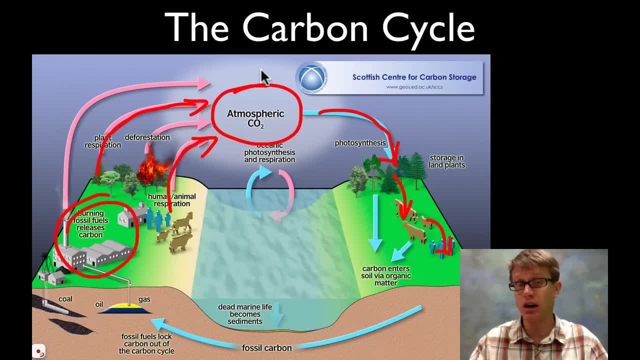 amount of carbon because we're burning fossil fuels, which releases more carbon than normally would be in the atmosphere. But we've got this wonderful recycling of carbon, And why do we need carbon Again to build us? Let's go to the next one, That's nitrogen. Why do 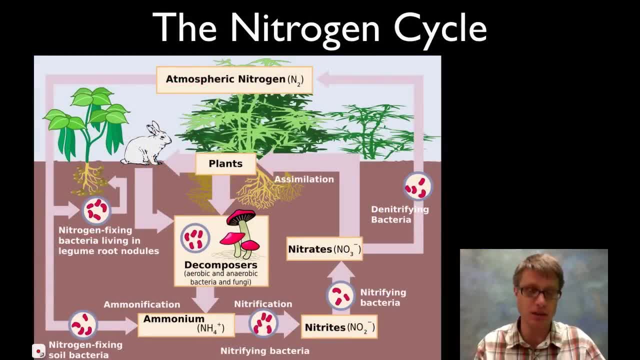 we need nitrogen. Remember amino acids and also the nitrogenous bases, Now the nitrogen cycle. basically, how do we move that into plants On the nitrogen cycle? on both sides we need bacteria And so in order to get it into plants, that nitrogen in the atmosphere. 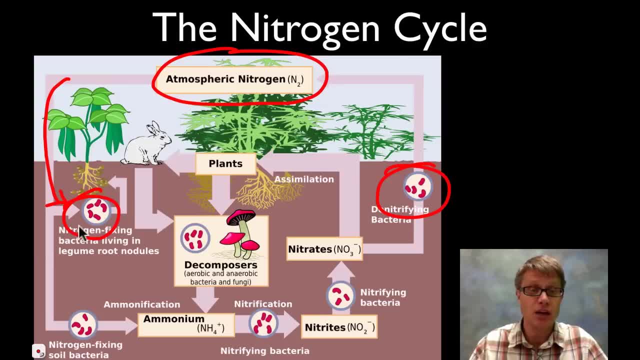 it's just nitrogen gas. 70% of what you're breathing now is nitrogen. In order to get that into plants, there are going to be bacteria And basically what they're going to do is fix the nitrogen. They're going to make it usable, And so, before a plant can absorb the 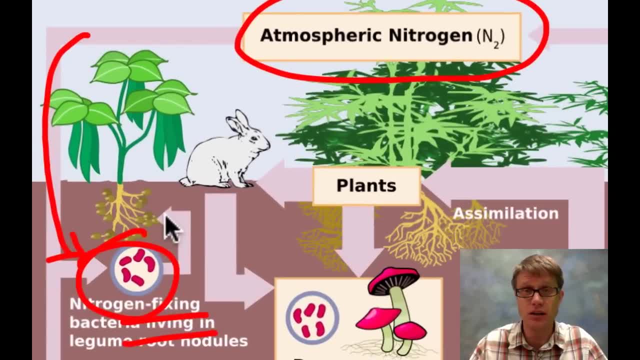 nitrogen. it has to be fixed, It has to be converted into nitrate And so, basically, bacteria are doing that And some plants will form a symbiotic relationship where they let bacteria live on their roots And they're going to be able to absorb the nitrogen And they're